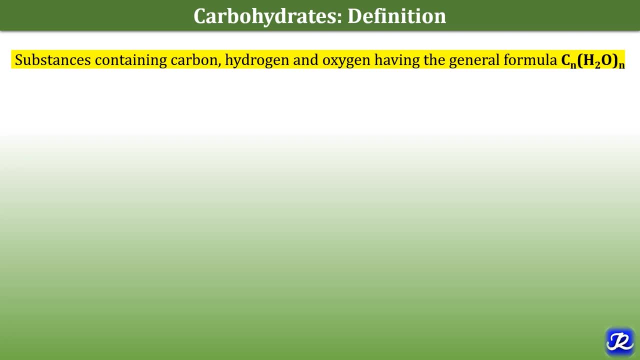 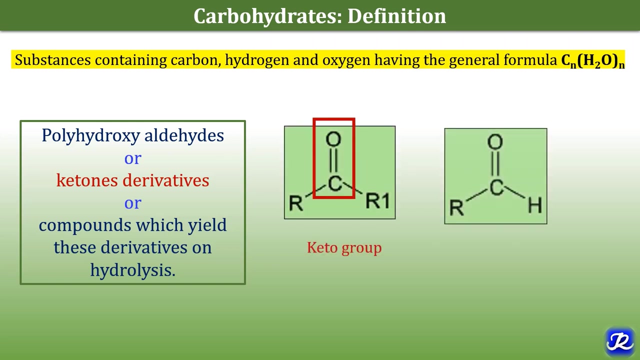 or sulfur. So what is the definition of carbohydrates? Carbohydrates are defined as polyhydroxyaldehydes or ketones or carbohydrates. Carbohydrates are the substances containing carbon hydrogen and sulfur and relate to other compounds which yield these on hydrolysis. What is mean by? 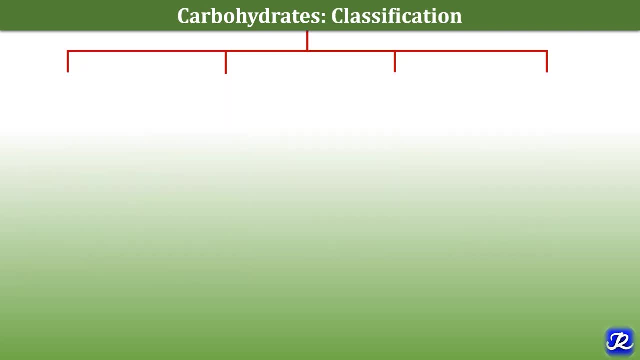 ketones, The compounds having these keto group, And what is mean by aldehydes, The compound having these aldehyde group. Carbohydrates are classified as monosaccharides means simple sugar. Sugar is soluble in water and sweet to taste. These monosaccharides they the simplest. 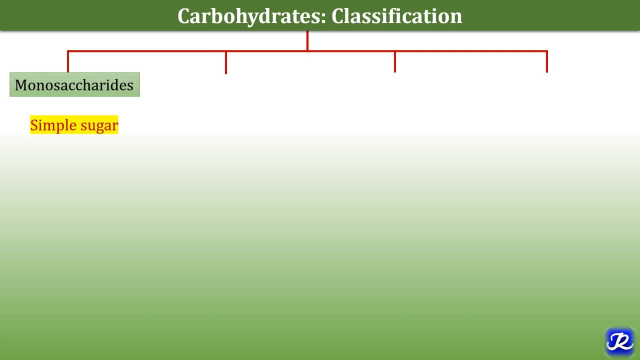 form of carbohydrates because they cannot be further hydrolyzed into simple formulae Review units. So this is the simplest form of carbohydrate: Disaccharides: they contain 2 monosaccharide units linked together by glycosidic linkage. Oligosaccharides contain 3 to 10 monosaccharide. 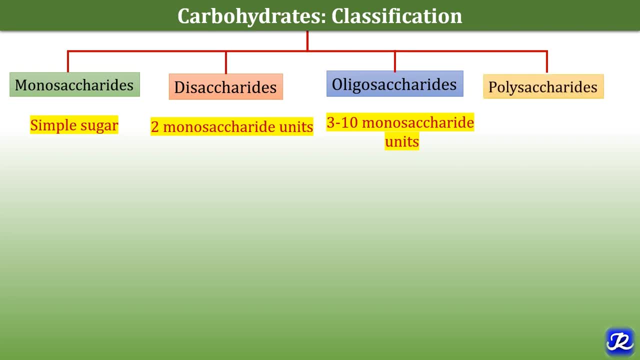 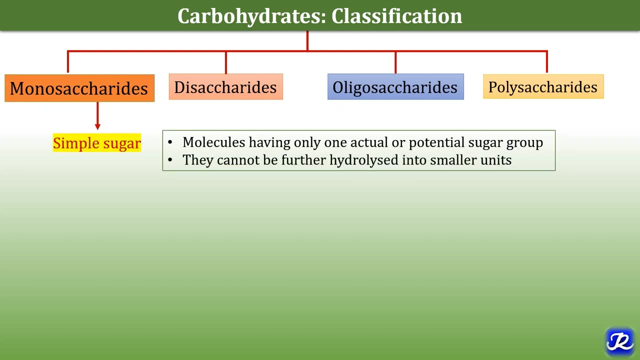 units joined together by glycosidic linkage And polysaccharides. they contain more than 10 monosaccharide units. Now let's talk about each group one by one. So first is monosaccharides. Monosaccharides are simple sugar and they are the molecules having one actual or potential 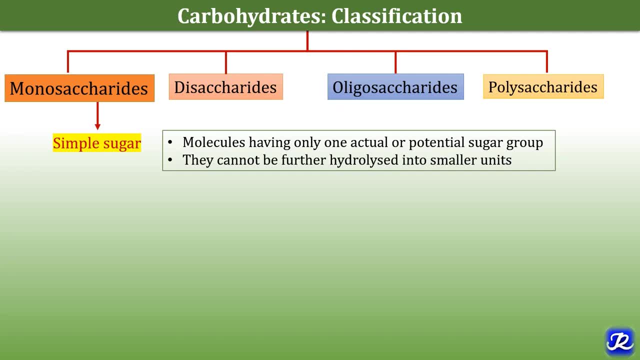 sugar group and they cannot be further hydrolyzed into smaller units. And these monosaccharides are further classified as aldoses and ketoses, and it depends on the presence of aldehyde group and ketone group. If the monosaccharide has aldehyde group, they are called as aldoses. 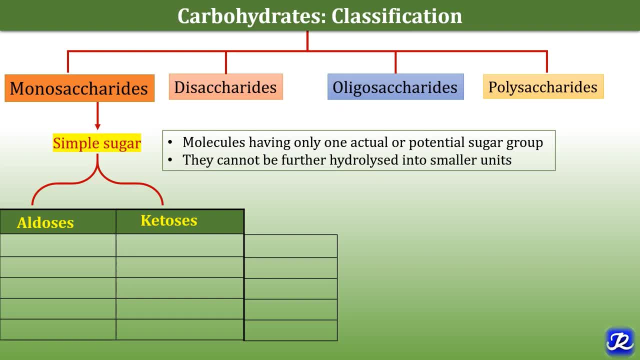 and if they have keto group, then they are called as ketoses. Now let's see the various examples. Glystraldehyde is aldo sugar and dihydroxyacetone is keto sugar. and both glystraldehyde and dihydroxyacetone, they contain 3 carbons and that's why they are also called as trioses. Erythrose is aldo. 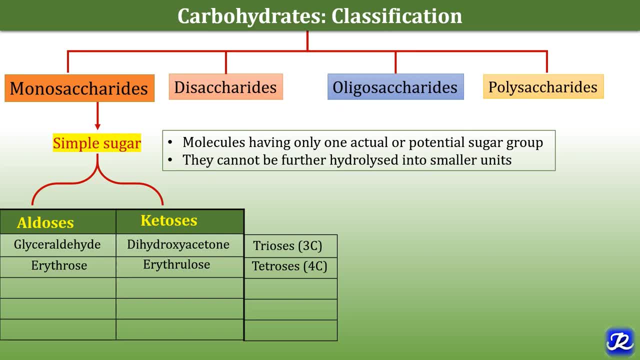 sugar. Erythrolose is keto sugar and they contain 4 carbons, so they are called as ketoses. Ribose is aldo sugar. Ribulose is a keto sugar, and both contain 5 carbons, so both are pentatonic. 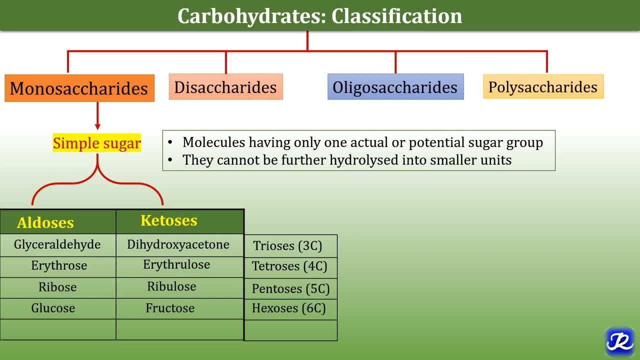 Glucose is aldo sugar and fructose is ketose, and both glucose and fructose they contain 6 carbons and that's why they are hexoses. Glucohepatose is aldose, Cedoheptulose is ketose, and both contain 7 carbons and that's why. 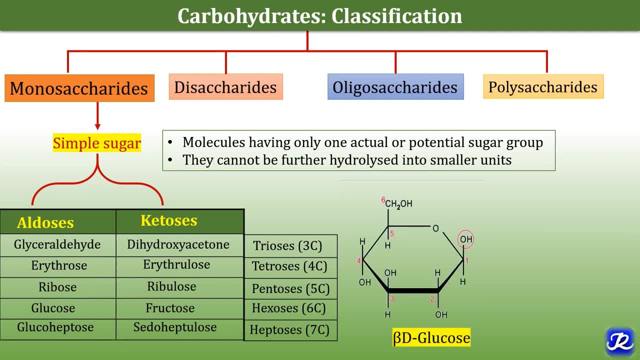 they are called as heptoses. This is the structure of beta D glucose. It contains 6 carbon and why it is called as beta D glucose. It contains 6 carbon and why it is called as beta D glucose. Beta means the hydroxyl group which is attached to carbon. 1. It lies above the plane of ring. 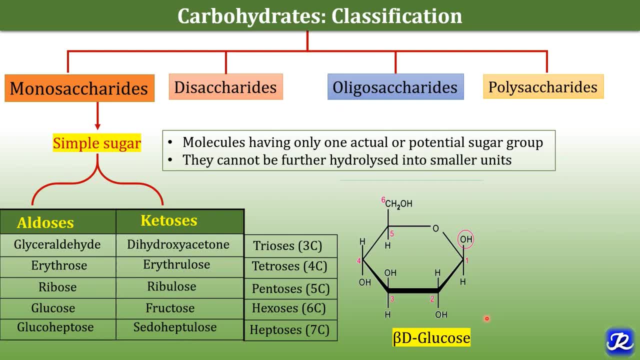 and that's why it is called as beta glucose, and D means it is a D isomer. Most of the monosaccharides in the living beings, they belong to D series and D glucose is the most abundant monosaccharide in nature And this is the structure of alpha D fructose. Why alpha? Because the hydroxyl group. 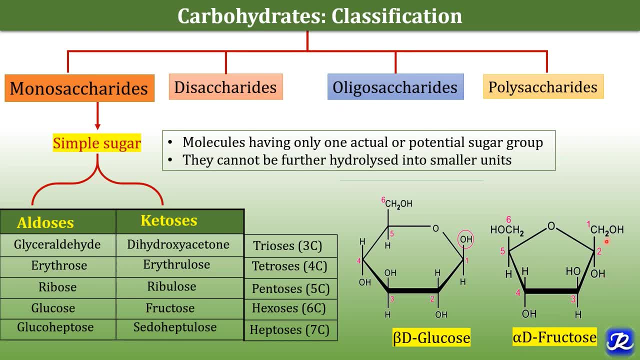 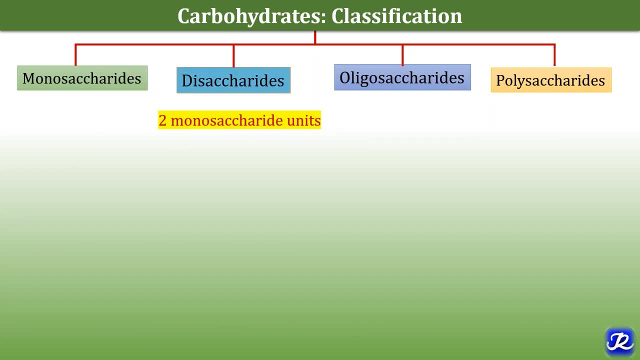 which is attached to the carbon 1, is called as alpha D fructose, And this is the structure of carbon 1.. It lies below the plane of ring and that's why it is called as. alpha Disaccharide contains 2 monosaccharide units, and these 2 monosaccharide units- they are linked. 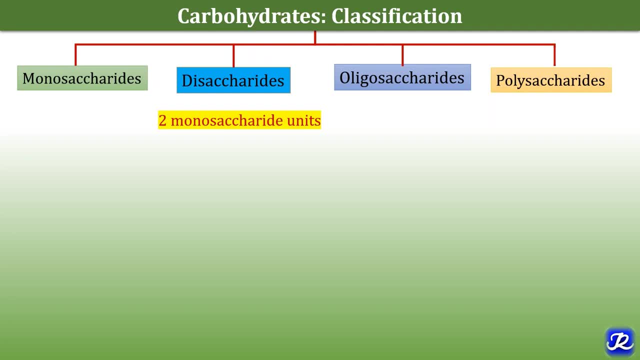 together by glycosidic bond, And disaccharides are crystalline and water soluble and sweet to taste, And they are further subclassified on the basis of presence or absence of free reducing group. So the disaccharides are classified as reducing. 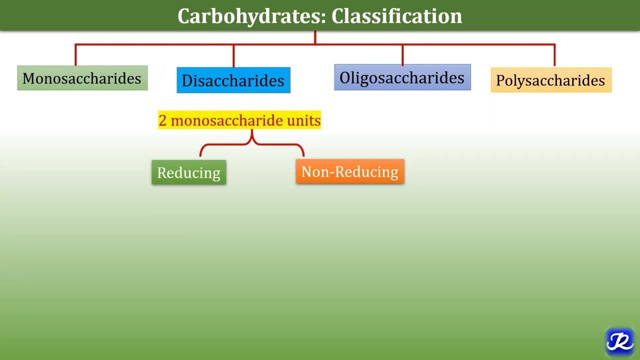 or non-reducing disaccharides. The reducing disaccharides examples are maltose and lactose. Maltose contains alpha D glucose plus alpha D glucose means 2 molecules of alpha D glucose. They are linked together by alpha 1,4 glycosidic bond. And what is the constituent of lactose? 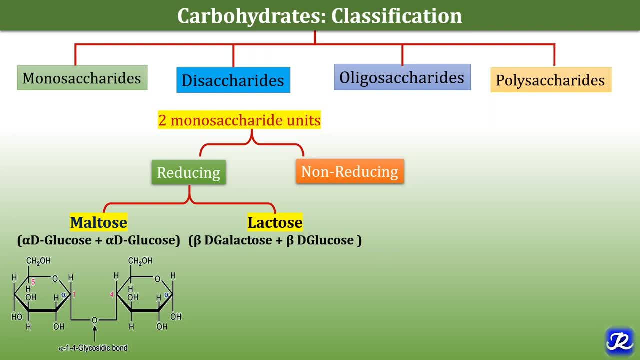 1 molecule of beta D lactose plus 1 beta D glucose. they are linked together by glycosidic bond To form lactose. So maltose and lactose. these are reducing disaccharides. What is the example of non-reducing disaccharide? It is sucrose. Sucrose is non-reducing disaccharide And it 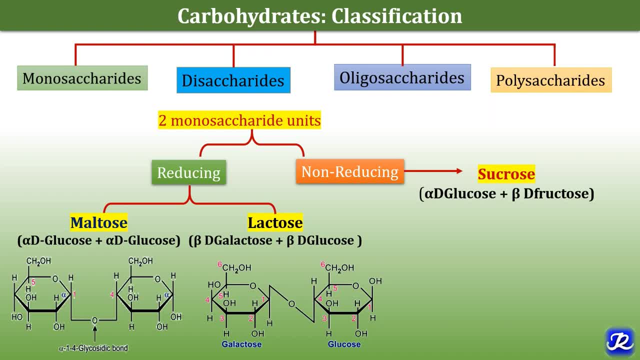 contains 1 molecule of alpha D glucose plus 1 molecule of beta D fructose And both molecules. they are linked together by glycosidic bond Oligosaccharides. they contain 3 to 10 monosaccharide units And they are linked together by beta D fructose, And they are linked together by 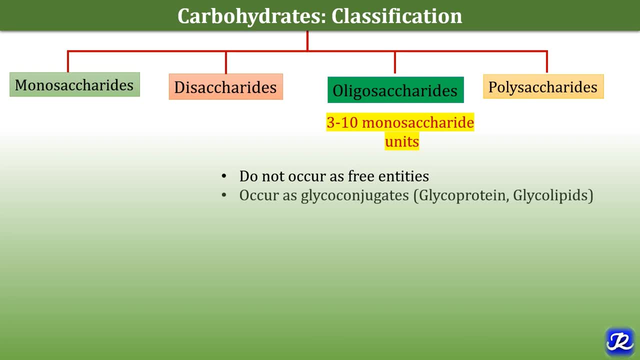 glycosidic bond. They do not occur as free entities in living beings and they occur as glyco conjugates, like glycoprotein glycolipids In plant world. the examples of oligosaccharides are raffinose, which contains 3 monosaccharide units, Like alpha D, glucose, beta D, galactose. 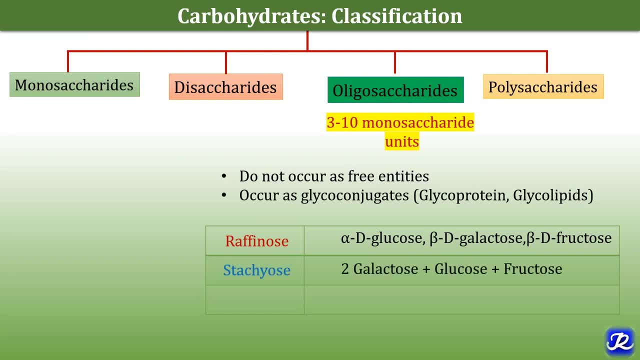 and beta D fructose. Stachyose is other example of oligosaccharide, which contains 4 monosaccharide units, 2 galactose, 1 glucose and 1 fructose. Verbacose: it contains 5 monosaccharide units, 3 galactose, 1 glucose and 1 fructose Raffinose. 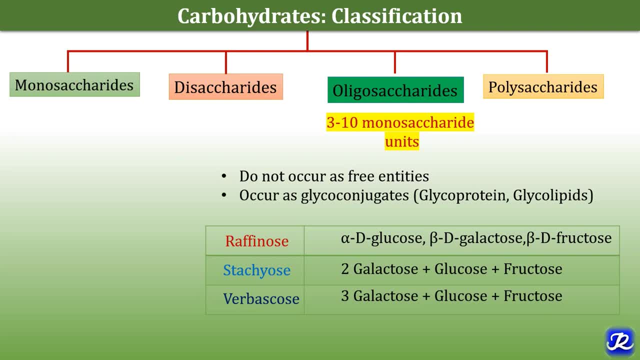 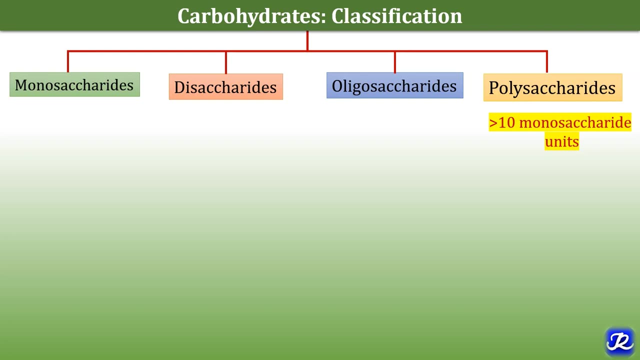 are present in beans, cabbage, broccoli, etc. Stachyose are also present in vegetables and plants. Verbacose they are present in legumes and they are fermented by intestinal bacteria and they cause flatulence. Coming to the polysaccharides, they contain more than 10 monosaccharide units. 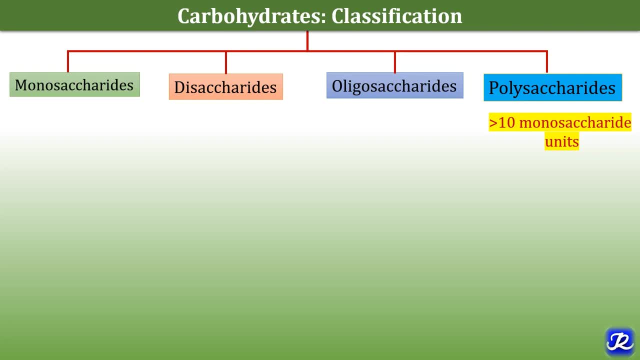 These polysaccharides are also called as Glycans or complex carbohydrates, and they have high molecular weight and we are sparingly soluble in water And they are not sweet in taste and do not exhibit any properties of aldehyde or ketone group, and they are further. 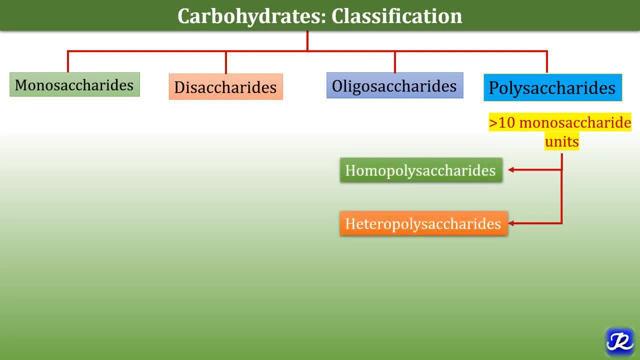 classified as Homo polysaccharides and hetero polysaccharides. Homo polysaccharides contain same type of monosaccharide units, and hetero polysaccharides contain More than or equal to two different types of monosaccharide units or their derivatives. 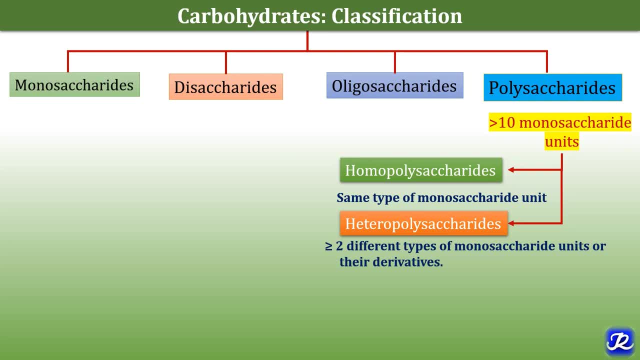 So polysaccharides are of two types: homopolysaccharides and heteropolysaccharides. Homopolysaccharides are also called as homoglycans and heteropolysaccharides are also called as heteroglycans. 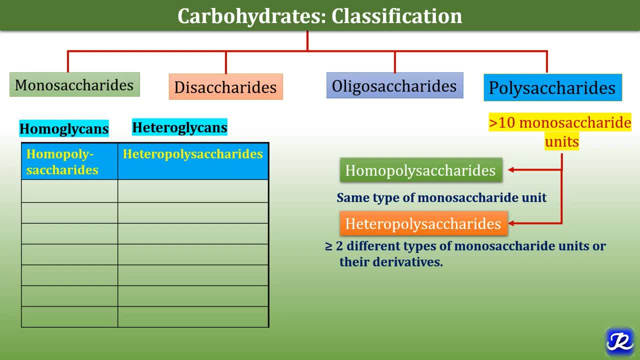 The examples of homopolysaccharides are starch, dextrin, glycogen, cellulose, inulin, dextran, chitin. And the examples of heteropolysaccharides are agar and agarose, gum and pectin and various GAGs like glycosaminoglycans, like hyaluronic acid, chondroitin, sulfate, keratin, sulfate, dermatin, sulfate, heparin, sulfate. 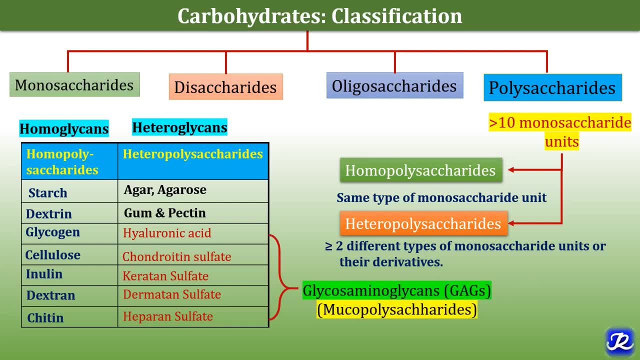 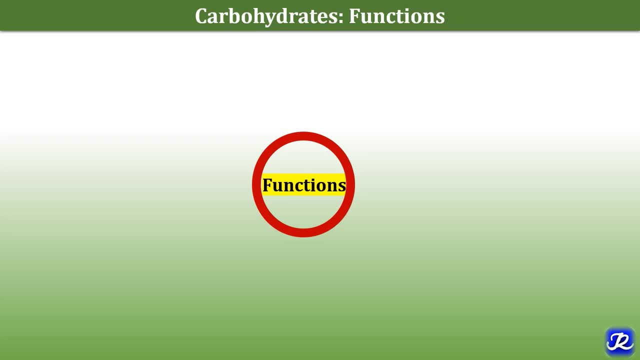 So these are called as glycosaminoglycans or GAGs, and earlier they were called as mucopolysaccharides. Now let's enumerate the functions of carbohydrates. They are the most abundant dietary source of energy. 4 kilocalories are formed when 1 gram of carbohydrate is oxidized. 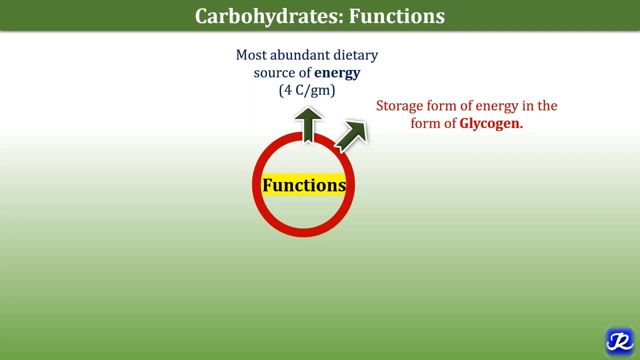 They are the storage form of energy in the form of glycogen. Glycogen is stored in the liver and muscle. The non-digestible carbohydrates like cellulose, agar, gum and pectin. they are dietary fibers. They are the precursor of organic compounds. 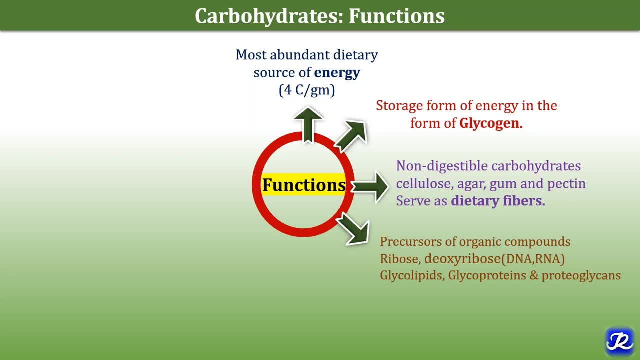 For example, ribose and deoxyribose. they are the important constituents of nucleic acids like DNA, RNA, And they are precursor of compounds like glycolipids, glycoproteins and proteoglycans. Carbohydrates participate in structure of cell membrane because glycolipids and glycoproteins are the constituent of cell membrane. 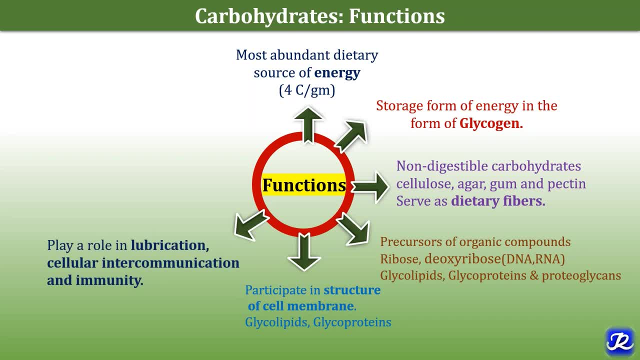 They play a role in lubrication because the GAGs, like hyaluronic acid, is important for lubrication of joints, cellular intercommunication and immunity. They serve as structural component, For example, glycosaminoglycans in humans, cellulose in plants and chytins. 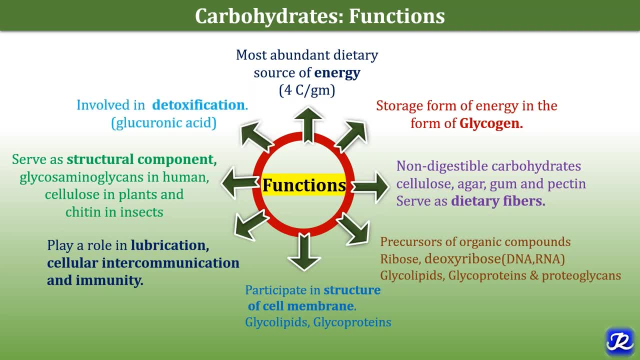 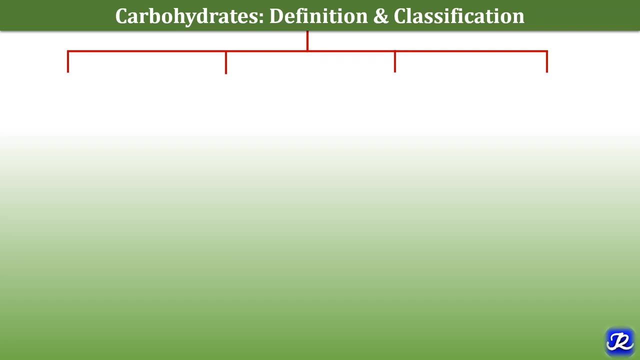 Glycosaminoglycans in insects, And they are involved in detoxification reaction. For example, derivative of carbohydrates, glucuronic acid, is involved in detoxification process. So let's now summarize the topic. Carbohydrates are defined as polyhydroxy aldehydes or ketones, or compounds which ill these on hydrolysis.